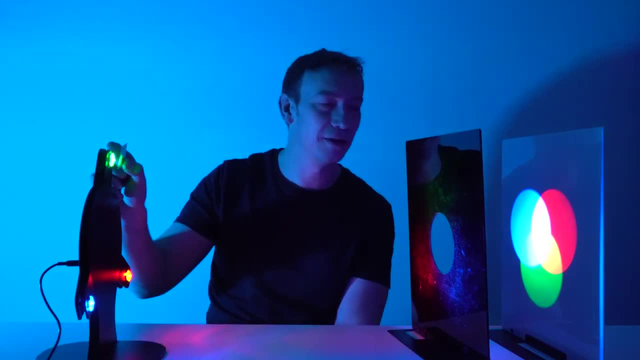 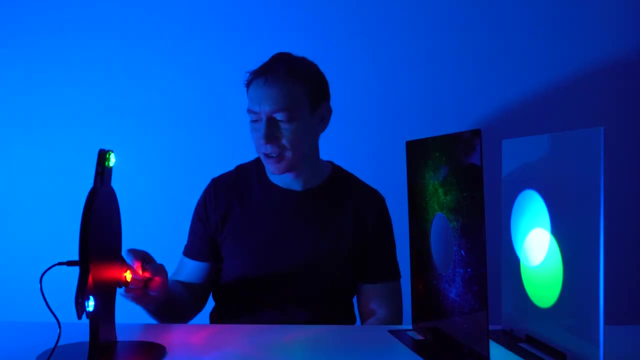 is a green filter. Now if I put it in front of the green light, it still lets the green light through because we can still see the green circle over here. But if I take that same filter and I put it in front of the red, it actually blocks out the red light. So 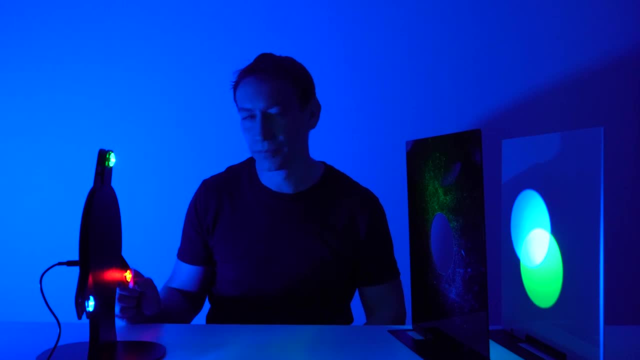 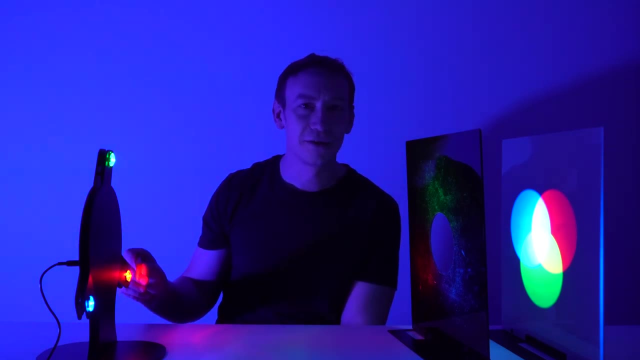 the green filter won't let red light through it. I've got another filter, This one's red, And if I put that red filter in front of the red LED now, we can see that the red light still gets through. And if I take that red filter and put it in front of the green, it absorbs all of the 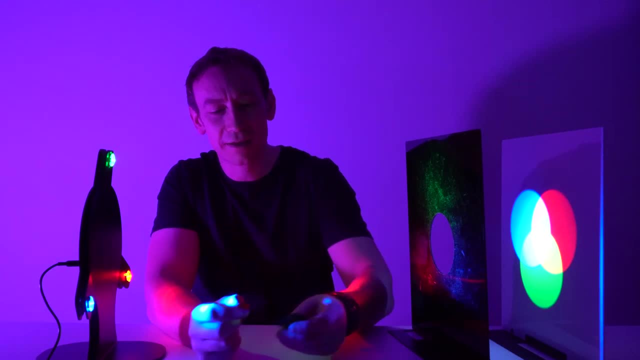 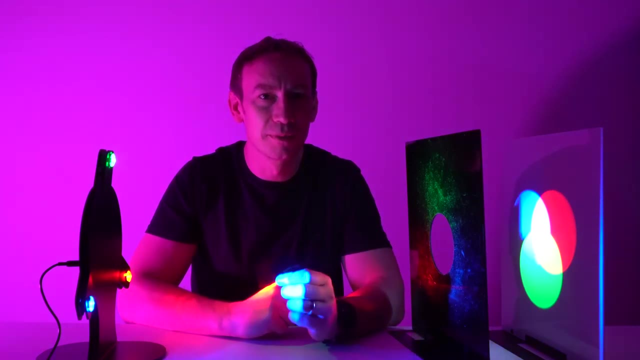 green light. So colour filters are useful And I suppose, depending on the colour filter, that tells you which colours of light it lets through and which colours are absorbed. So I've got four objects here, but what colour are they? Well, with a red filter, we appear. 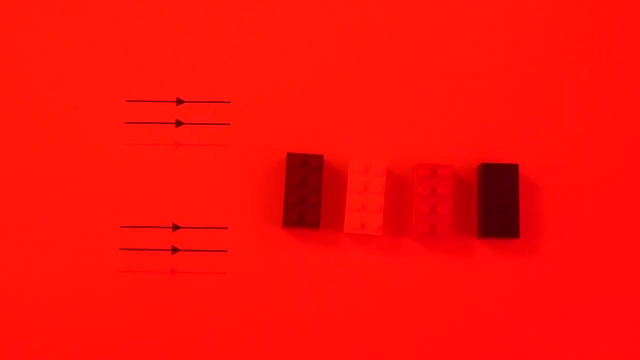 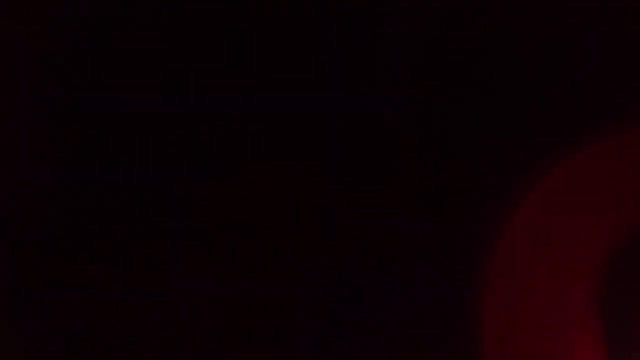 to have a dark object, two lighter coloured objects and a dark object. If I then have a blue filter as well, if I hold this in front of the red filter, it actually filters out the light and we can't see anything. But if I sort the filters over and we look at this, 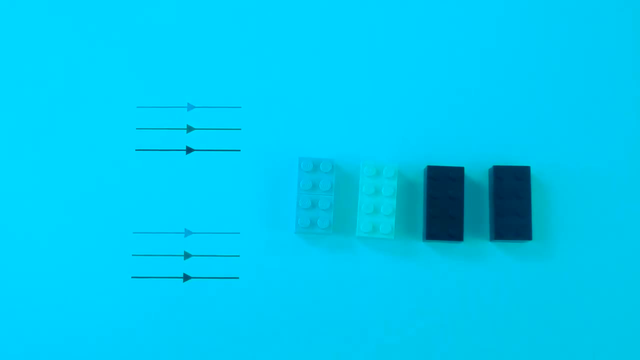 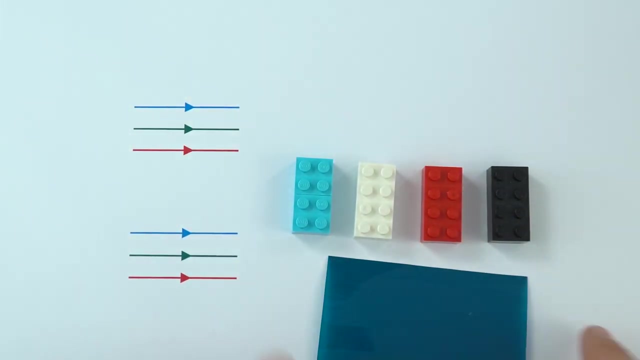 through a blue light. we've got two light coloured objects and two dark objects. So what colour are they? Well, we actually have blue, white, red and black. Now, a blue filter works by allowing the transmission of blue light, but it absorbs all the other. 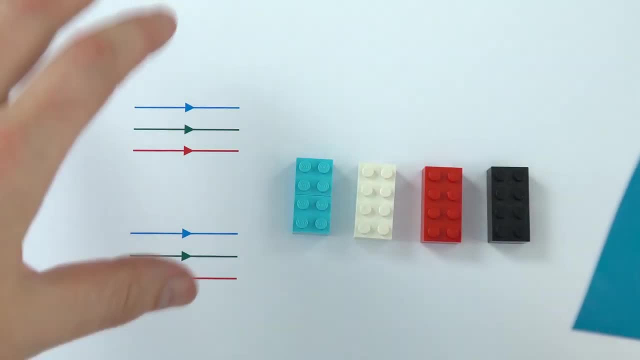 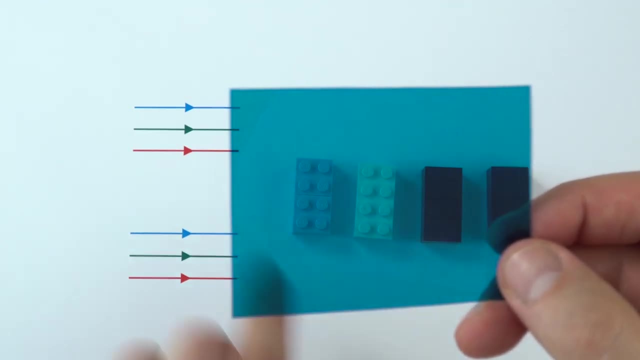 colours of light. Now, what that means is there's white light landing on this paper at the moment and the paper's reflecting all the colours of light. So if I take that light now, if I have a blue filter over a white object, the filter filters out all the 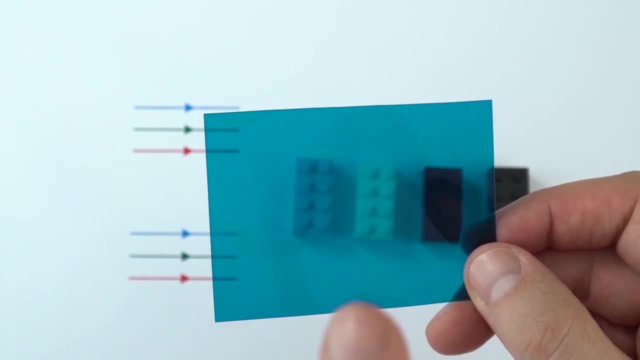 colours of light, and it only lets the blue light from the object get through the filter up to the camera. The blue object is only reflecting blue light, and that blue light comes through as well, so therefore it appears to be not that dissimilar to the background. 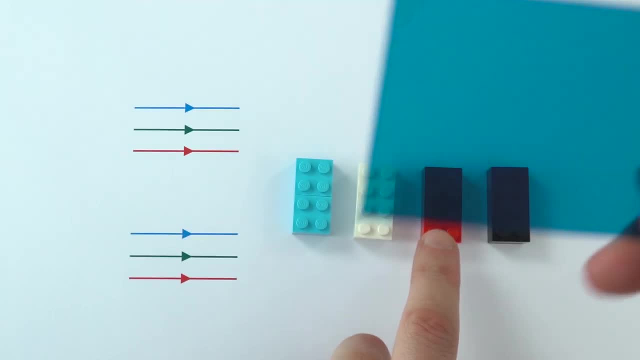 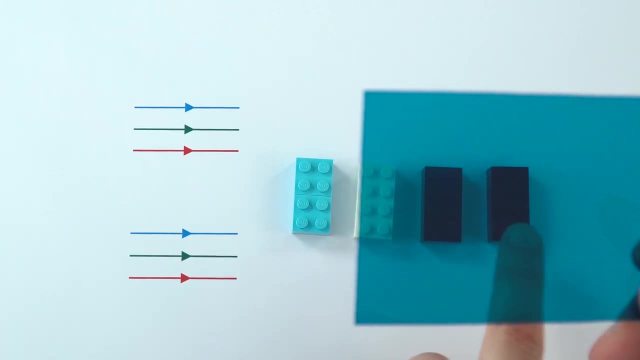 But if I have a red object, this is reflecting red light and the red light doesn't get through the blue filter and therefore it all appears to be black. In actual fact, through the filter, they both appear equally as dark, even though one is red and one is black.